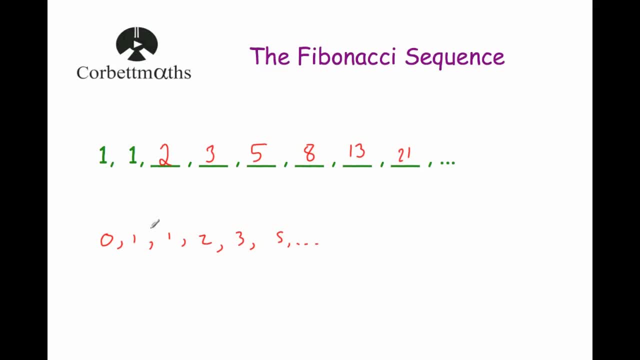 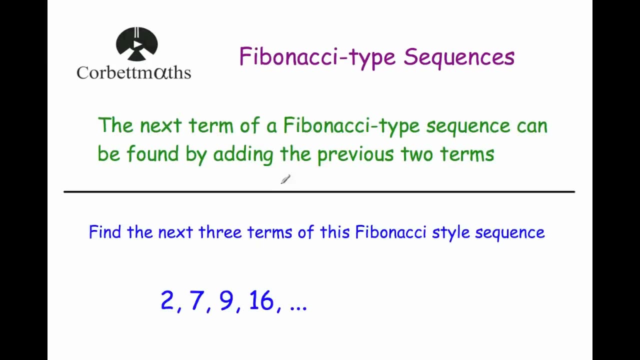 the top. I like that one. Sometimes you might see a zero at the front of it, sometimes you might not. Okay, So that's Fibonacci sequence and these Fibonacci numbers. Let's look at Fibonacci style sequences. So the next term in a Fibonacci style sequence is just found by adding the two previous terms. 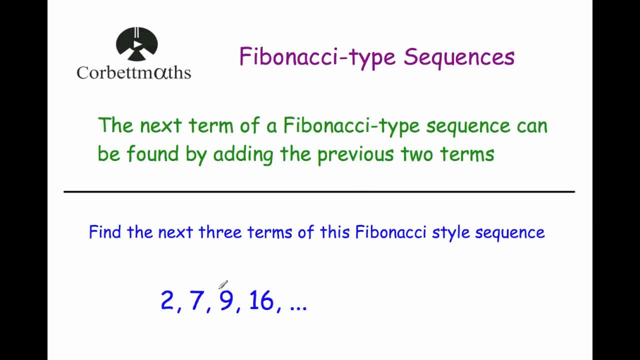 So in the same style, but just not with the numbers one on one. it could be other numbers. So here we've got a Fibonacci style sequence. So two plus seven is nine, seven plus nine is sixteen. We've been asked to generate the next three numbers to find the next three. 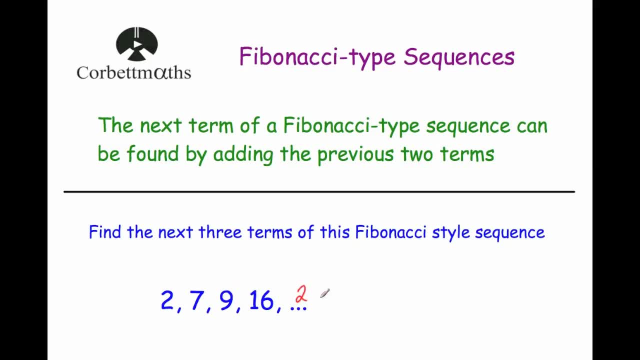 terms plus 16,. well, 9 plus 16 is 25,, 16 plus 25 would be 41, and 25 plus 41 would be equal to 66.. So they would be the next three terms in that Fibonacci style sequence. So you just. 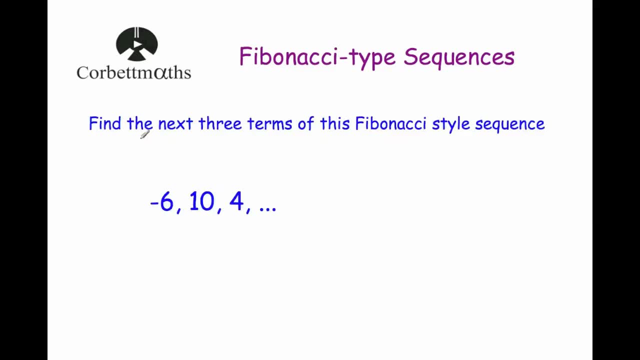 add the two previous numbers. Okay, next question. Our next question says: find the next three terms of this Fibonacci style sequence. So we've got negative 6 plus 10, so negative 6 plus 10 is 4.. So then 10 plus 4 is equal to 14,, 4 plus 14 is equal to 18, and 14 plus 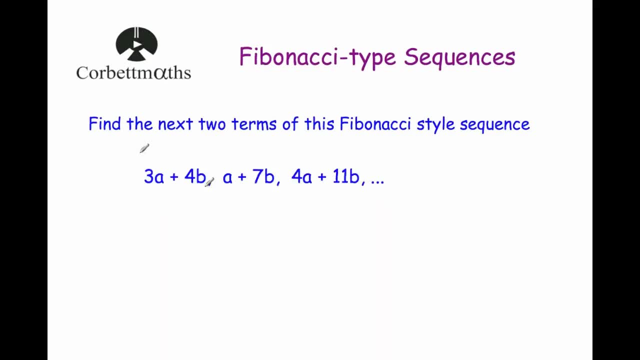 18 is equal to 32, and so on. So our last example says: find the next two terms of this Fibonacci style sequence, And the first three terms are 3a plus 4b, a plus 7b, 4a plus 11b. 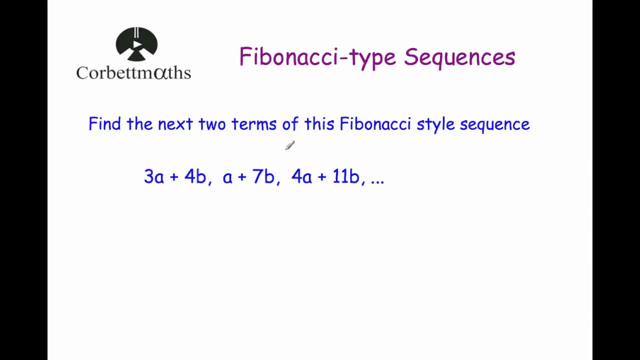 So let's just check and see how that was generated. So 3a plus a is 4a and 4b plus 7b is 11b. So let's find our next term. So we'd add these two terms together, the a plus 7b, and 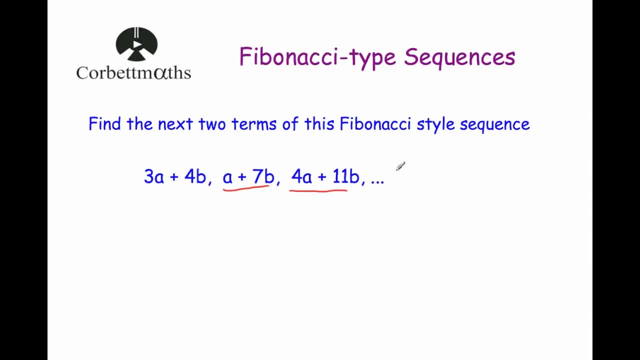 the 4a plus 11b. So a plus 4a would be 5a plus 7b plus 11b would be 18b. So that's the fourth term. And finally, the fifth term would be: 4a plus 5a is 9a, and 11b plus 18b would. 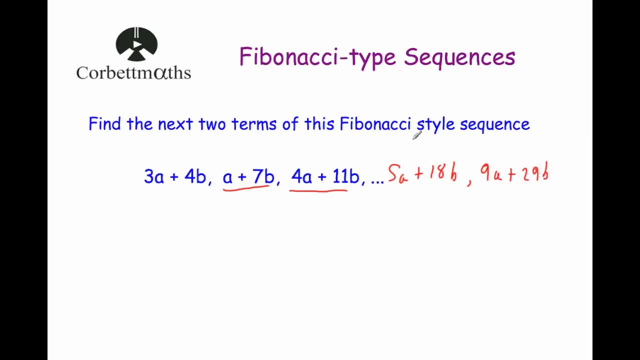 be 29b, And that's it. So Fibonacci style sequences can lead themselves quite nicely to algebra questions like this. But just remember: to generate a Fibonacci style sequence or Fibonacci type sequence, just add together the two previous terms to get the next one, and so on.